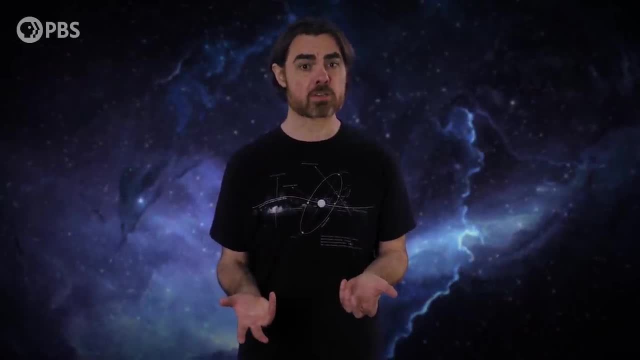 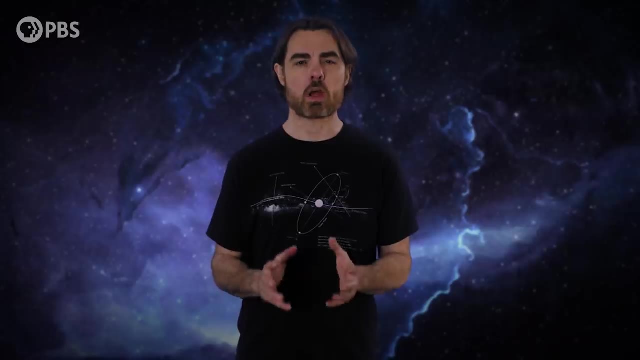 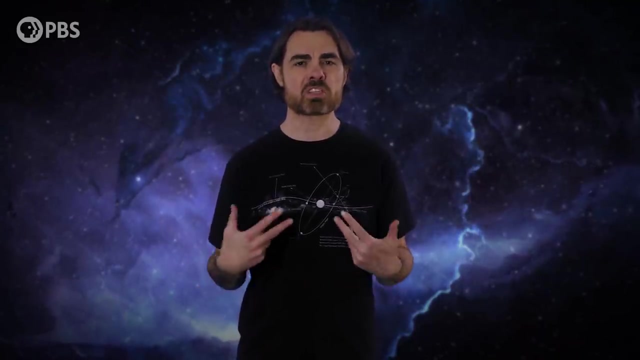 between light and gravity. Or is truth in fact entirely relative? Gravity bends the path of light. That fact is guaranteed by Einstein's general theory of relativity, But for some reason we scientists have been convinced of the fact with no good. 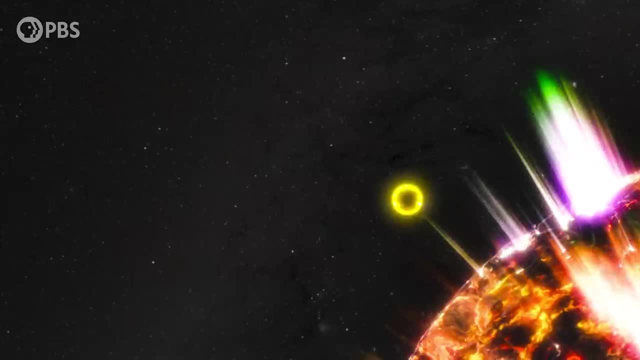 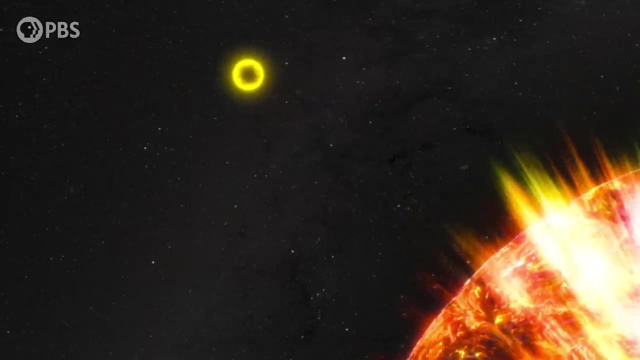 evidence for hundreds of years. In 1783, the English clergyman John Mitchell proposed that a particle of light gripped by the gravitational field of a sufficiently massive star would slow down, stop and fall back, And so was the first to predict the existence of light. 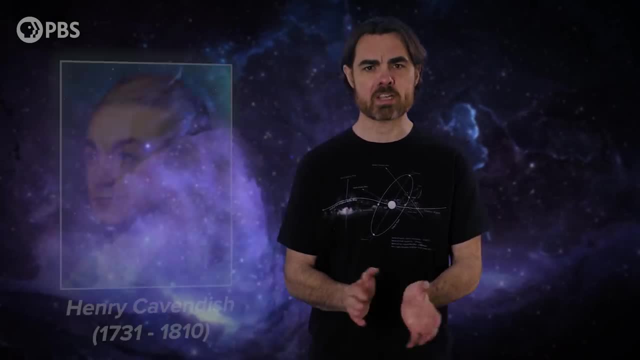 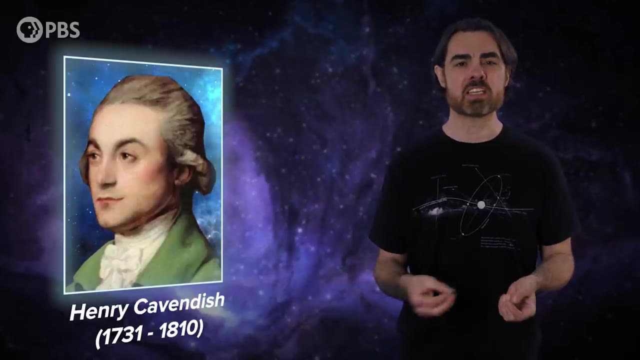 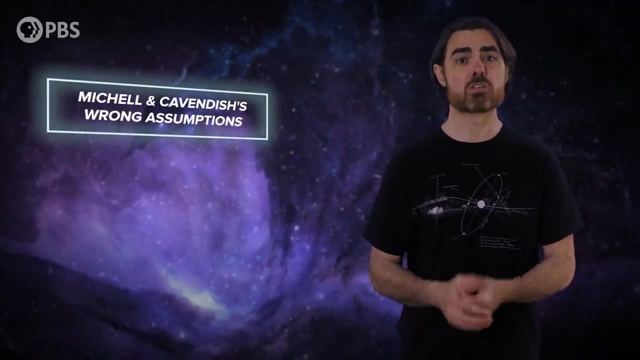 Mitchell wrote to his good friend Henry Cavendish on the subject, and Cavendish followed similar reasoning to predict that a particle of light would be deflected in its path as it passed near a massive object. Mitchell and Cavendish used the same utterly wrong assumptions to 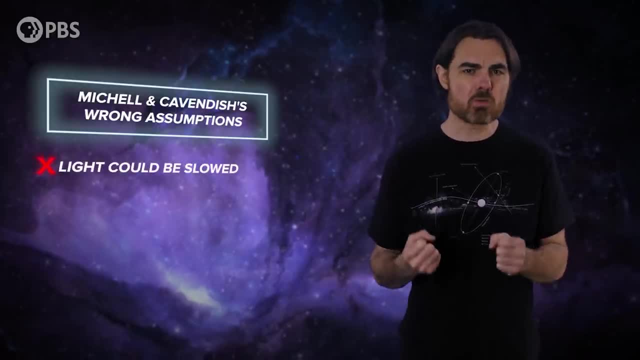 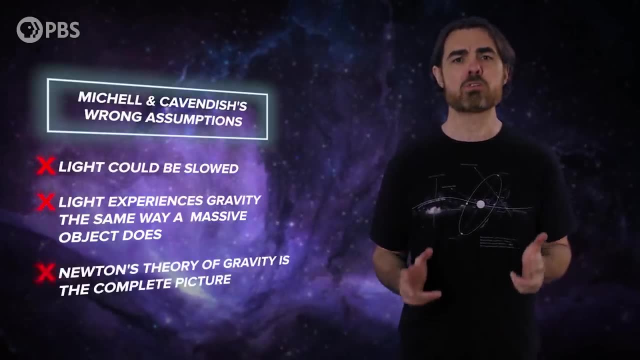 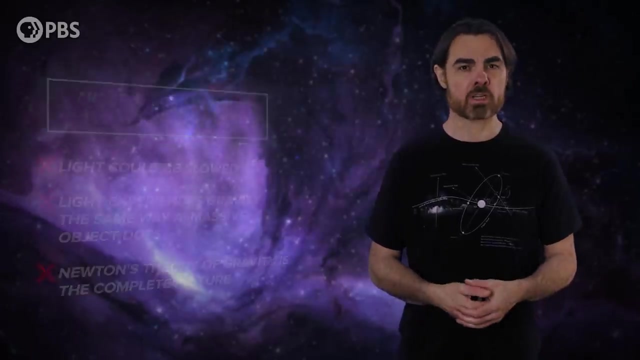 do their calculations. They assumed that light could be slowed down and that light experiences a force of gravity in the same way that a massive object does. They assumed that Isaac Newton's theory of gravity was the full picture And that light behaves like any other particle in response to Newtonian gravity. 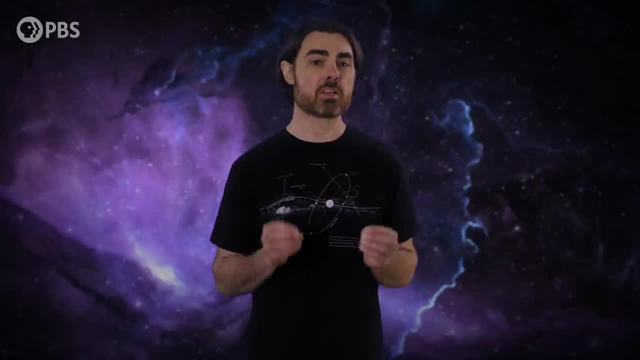 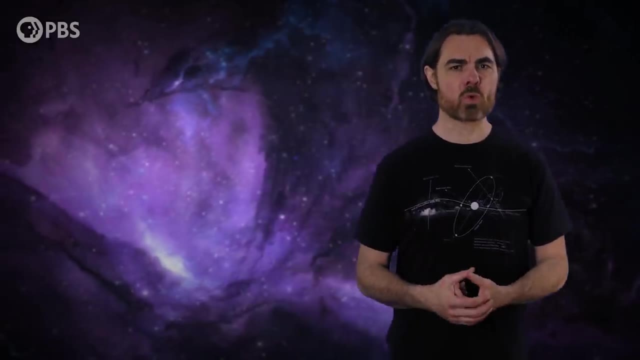 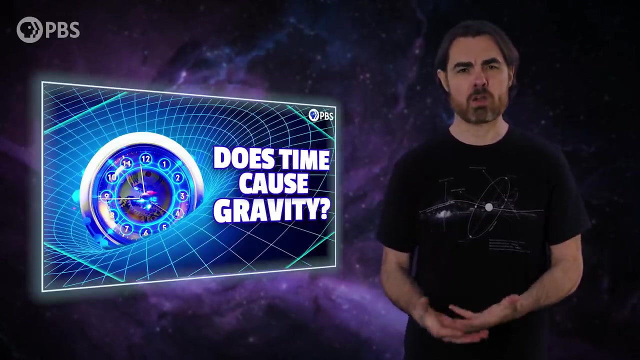 But the weird thing is that, despite these incorrect assumptions, the effects that these guys predicted have proved very real. We now know that both gravity and light are much weirder than Newton thought. We explored some of this in recent episodes, when we saw that what we experience as a force of gravity 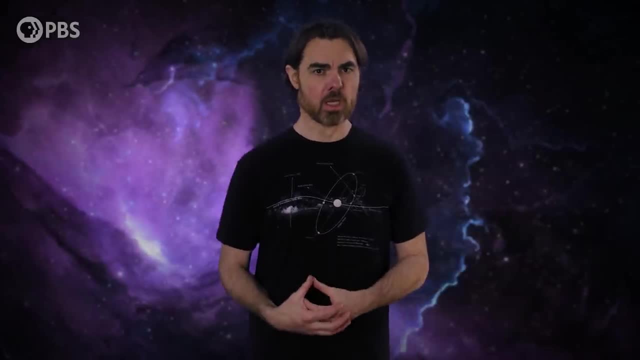 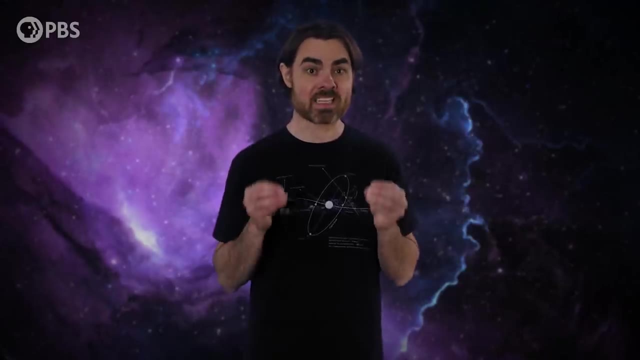 is mostly due to the way mass warps the flow of time. But the photon doesn't experience the flow of time, It doesn't even have any mass, And yet general relativity demands that gravity does affect light in ways eerily close to. 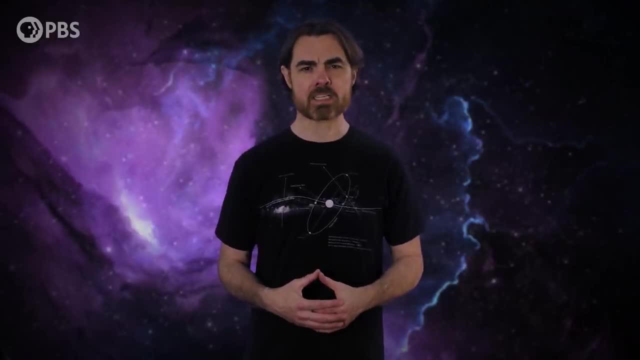 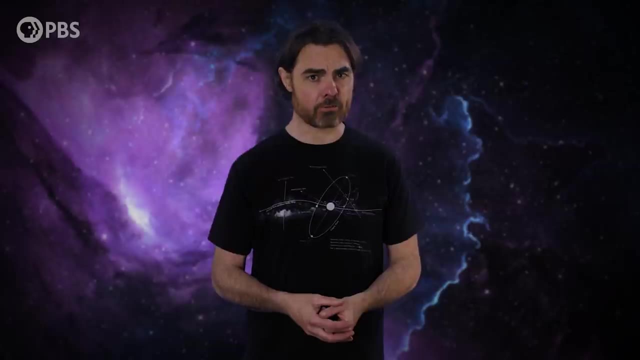 the predictions of Mitchell and Cavendish. The really hard part is understanding the why of it. What is really happening when light interacts with gravity? Let's see. if we can't figure it out In general relativity, the best place to start is always the equivalence principle. This: 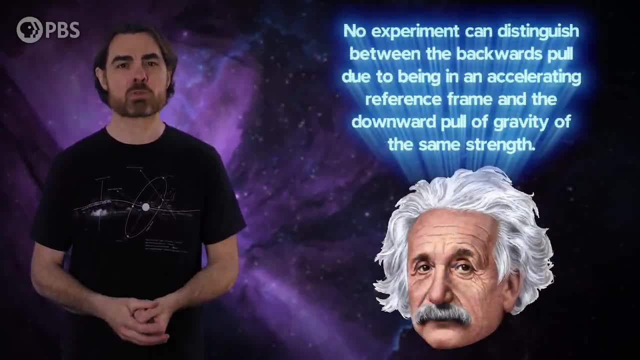 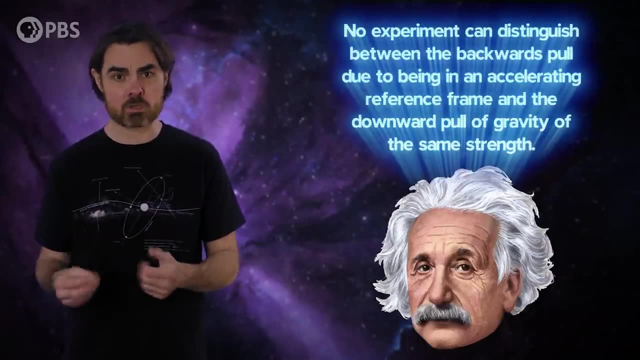 is Einstein's great insight that there's no experiment that can distinguish between the backwards pull due to gravity and the backwards pull due to mass. This is an example of the difference between being in an accelerating reference frame and the downward pull of gravity of the same strength or of the sense of weightlessness. 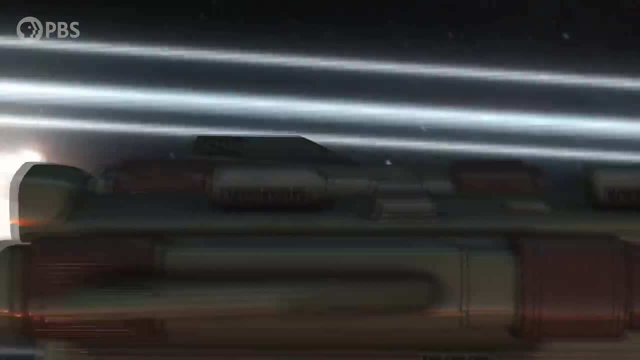 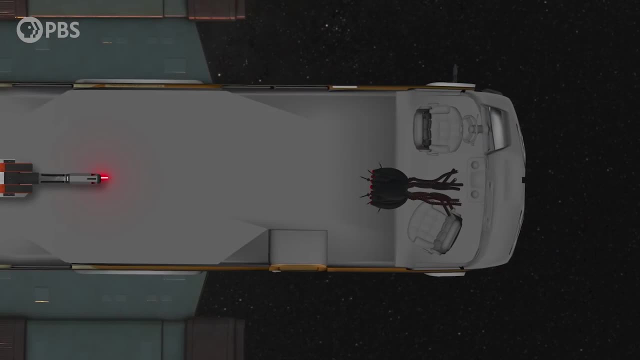 in freefall in a gravitational field versus the weightlessness felt in the absence of gravity. Imagine that you're in a rocket ship, accelerating rapidly to escape giant alien spiders or something. A spider breaks through the front hull and you fire your laser at it By the 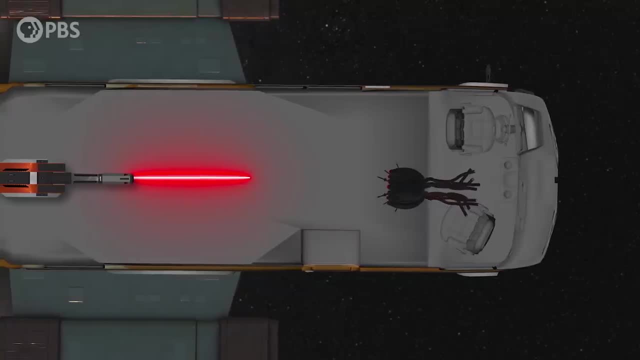 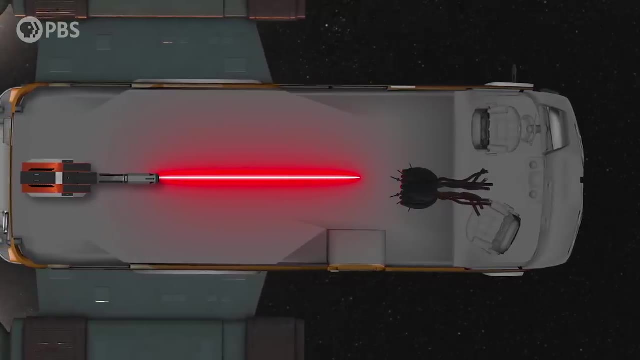 time the beam reaches its target, the ship is moving a little faster than when it fired. observe as the laser traveling at the speed of light, because the speed of light is invariant to all observers. but something else does change. See, light is a wave. 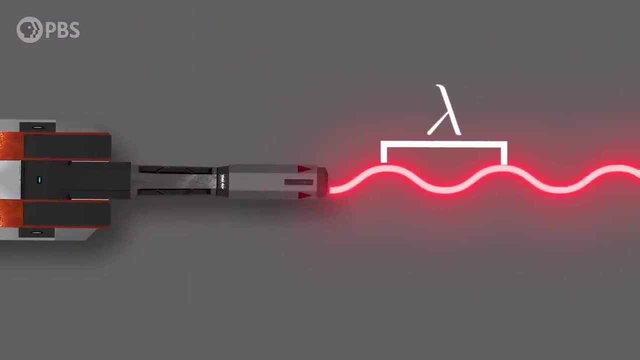 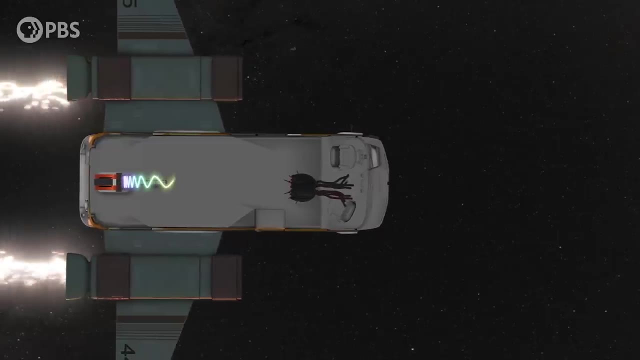 The distance between the peaks of that wave is its wavelength. After the front peak of your laser pulse reaches the spider, the ship continues to accelerate, which means the second peak has a little further to travel than the first And the third peak further still. 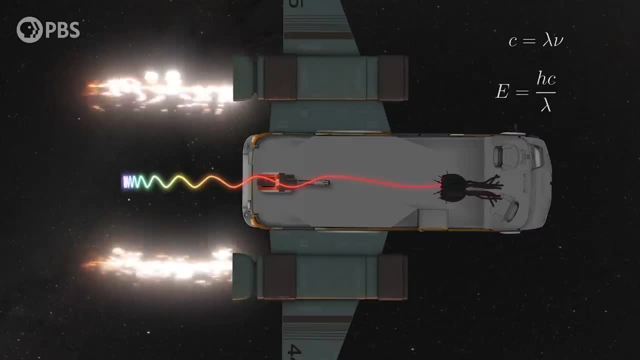 The distance between the peaks gets drawn out, wavelength increases, which means frequency and energy drop. Your laser power rating goes from kill to tickle. Good news for the giant alien spider, not so much for you. The equivalence principle tells us that we must experience all the same physics if at 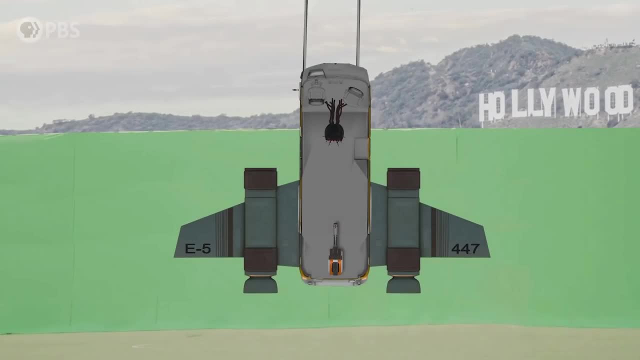 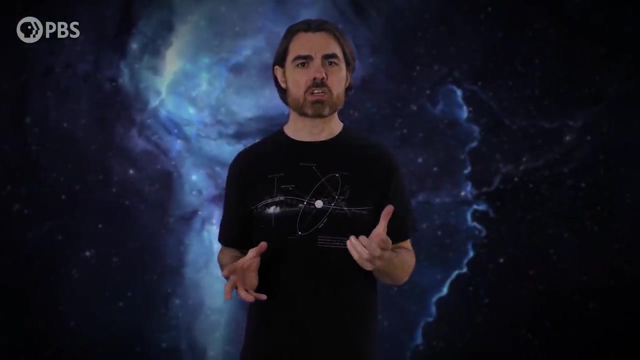 rest in a gravitational field, say in a fake rocket ship in a Hollywood set that for some reason is also being attacked by giant alien spiders. Light emerging from a gravitational field is stretched out, It experiences gravitational redshift, And we get exactly the same prediction if we use the fact that time runs slow in gravitational 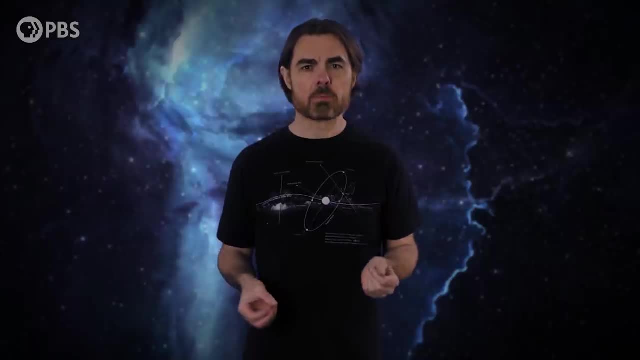 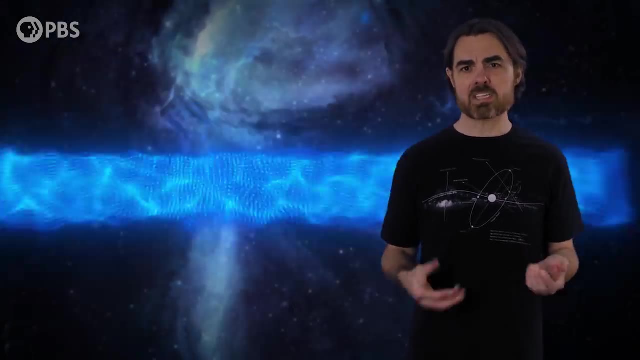 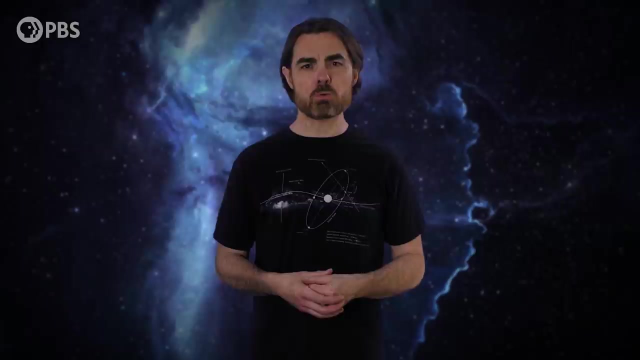 fields. Any process that generates a photon of light can be thought of as a clock, be it an electric charge pulsing up and down in a radio antenna or an atom vibrating back and forth in a glowing light filament due to its heat. These are the ticks of a clock and the frequency dictates the frequency and wavelength of the. 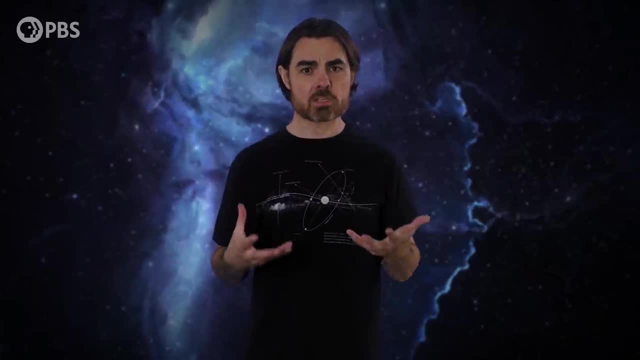 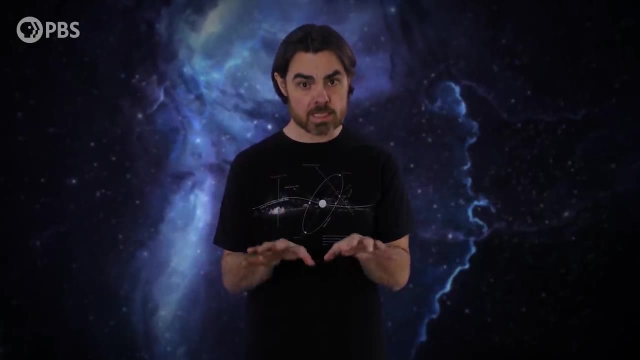 photon produced by that motion. But from a great distance away, Those clocks appear to run slow, and so the frequency of light emerging from within a gravitational field is lower, And if the density of the gravitating body is large enough, light emerging from it can. 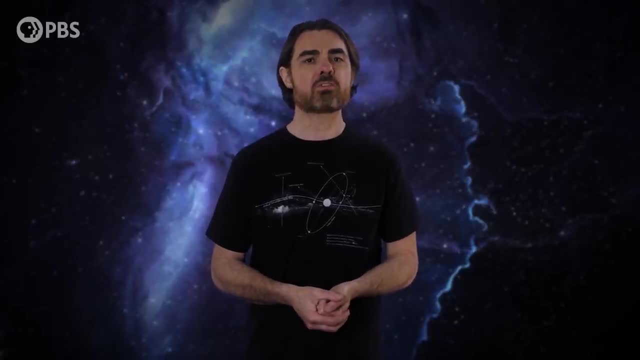 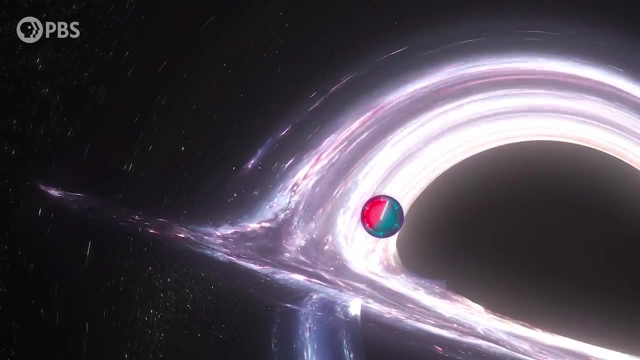 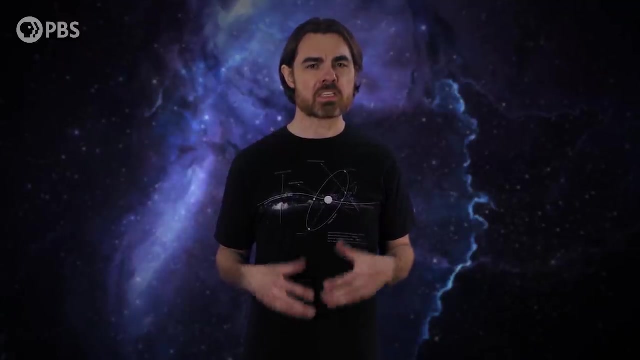 be sapped of all energy redshifted. so the wavelength is effectively infinite. At the event horizon of the black hole, gravitational time dilation is so strong that clocks stop and the frequency of photons trying to escape is brought to zero. The star thing is that the density of mass required to produce this infinite redshift 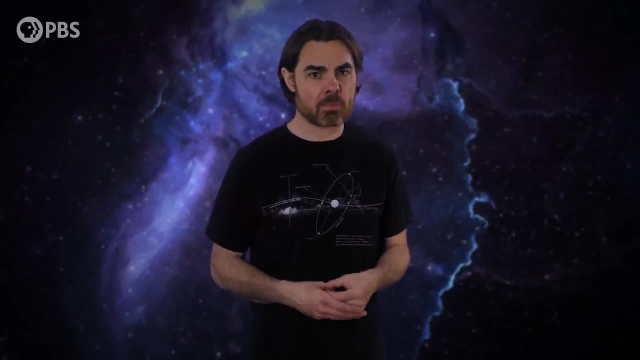 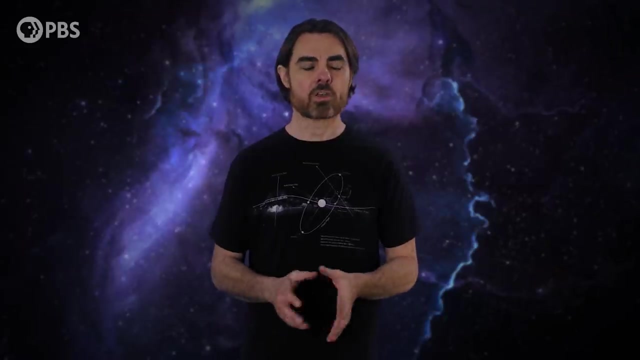 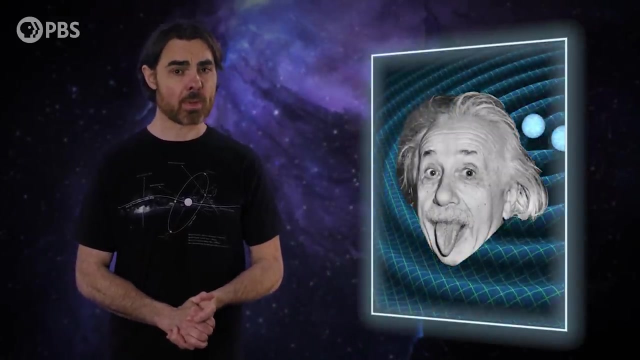 is exactly the same as is required to turn a light-speed particle around and have it fall back, as calculated by Mitchell from totally wrong assumptions. OK, let's tackle an even trickier problem, the solving of which shot Einstein to his international fame in talking about the deflection of the path of light by gravity. 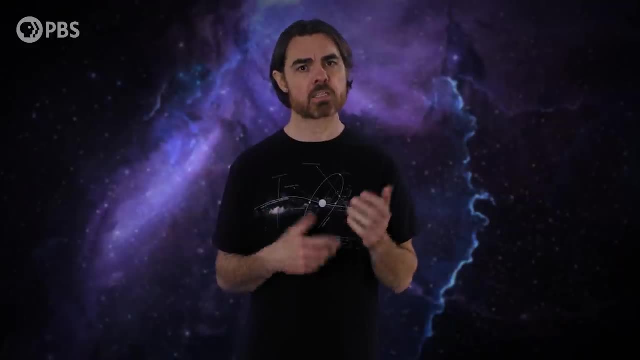 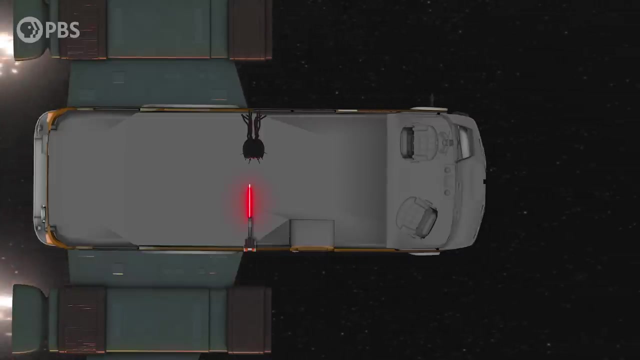 Let's start with the good old equivalence principle. again. And a spaceship attacks a star. This time you fire your laser across the deck perpendicular to the direction of acceleration. If you aim straight, do you hit? Let's look at it from the perspective of a non-accelerating observer outside the ship. 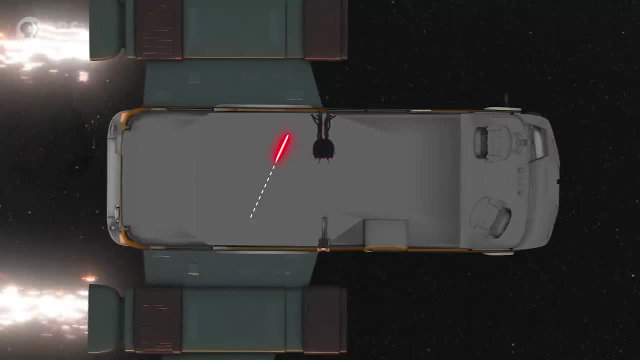 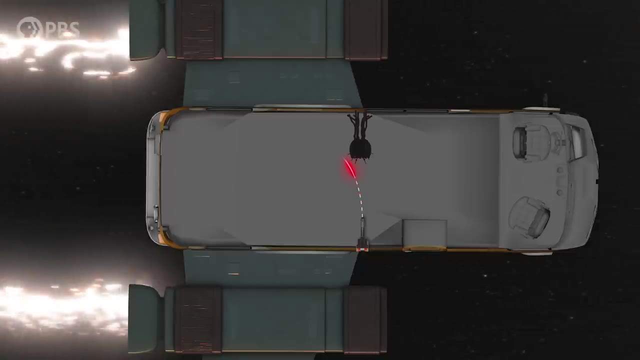 They have to see light travel in a straight line in the absence of any gravity. But for that to be the case, light must travel a curved path. from the point of view of the accelerating frame, You aim straight but miss your mark. These giant alien spiders are no joke. 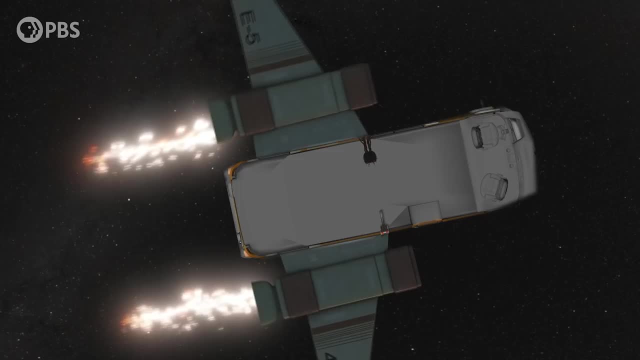 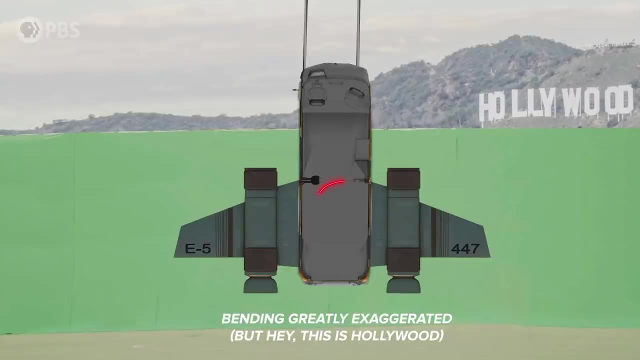 And the equivalence principle tells us that we must see the same bending of the light ray in our stationary rocket ship set in our gravitational field. OK, so that's the prediction. In the case of gravitational redshift, we could come up with a physical explanation. 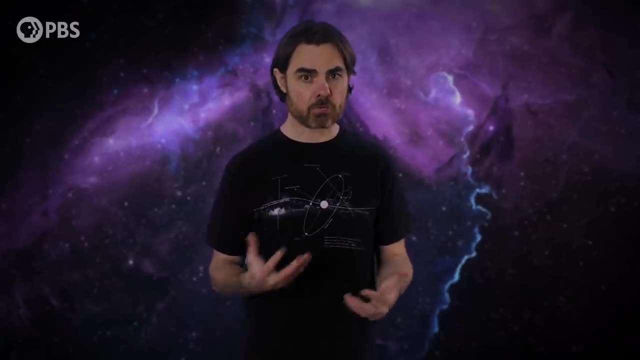 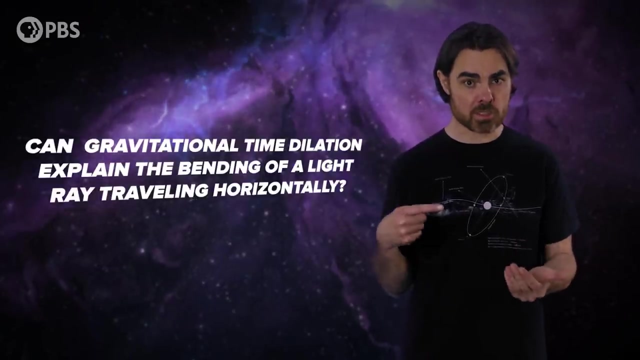 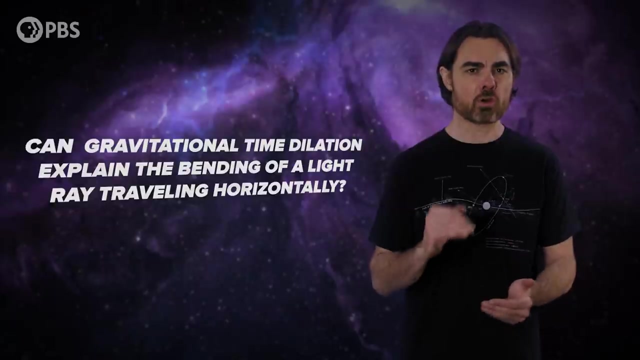 for the prediction. The difference in the flow of time changes the frequency of outgoing light. Can this gravitational time dilation also explain the bending of a light ray traveling horizontally? Well, tricky, Because there's no change in clock speed in the horizontal direction, only in the vertical. 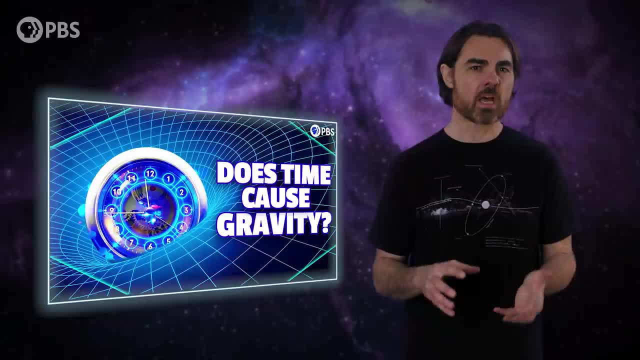 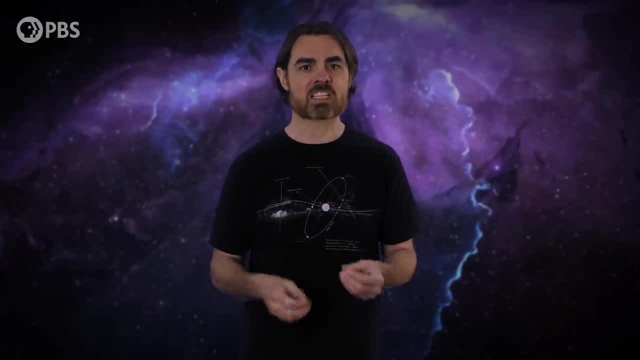 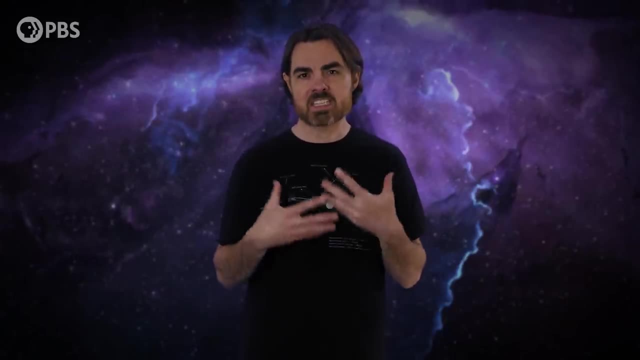 But we saw in our previous episode that a gradient in clock speed across the vertical extent of an object is enough to drag it downwards. To get technical, any massive object has a component of its four-dimensional spacetime velocity. in the time direction That temporal component is rotated into the downward spatial direction, which translates: 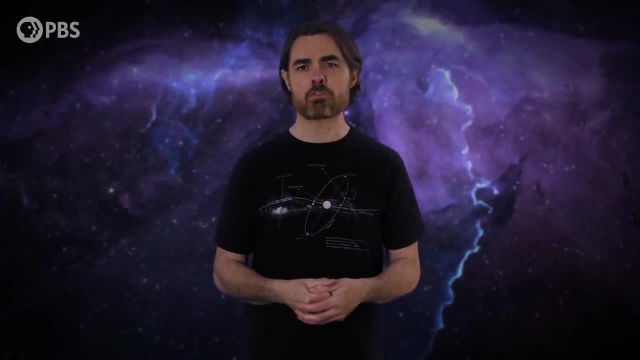 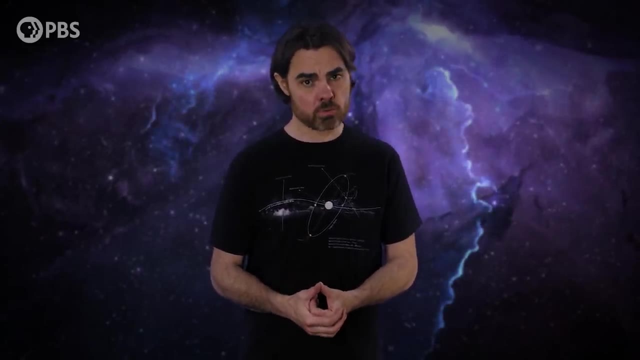 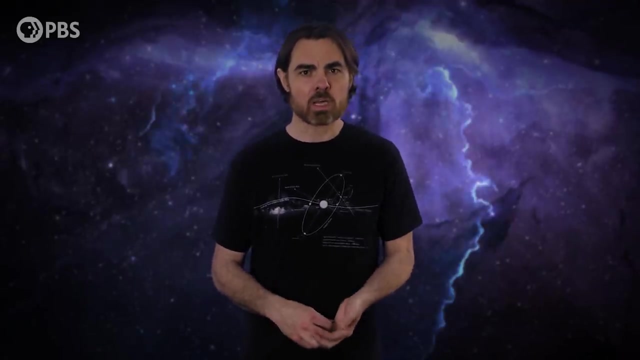 Well, that's the question- Into falling. But light is frozen in time. from its point of view, It has no time component to its velocity. It has in fact no time to lose. So if we imagine light as a perfectly narrow ray, or even as a massless, timeless particle, 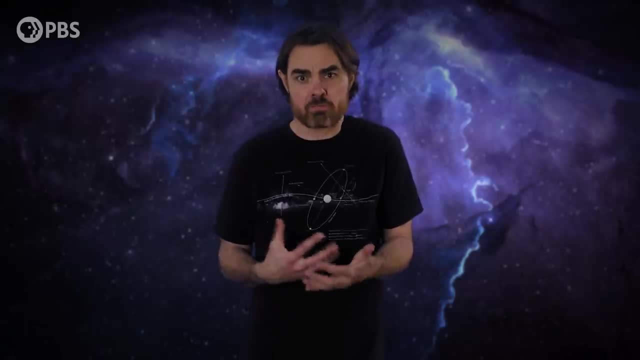 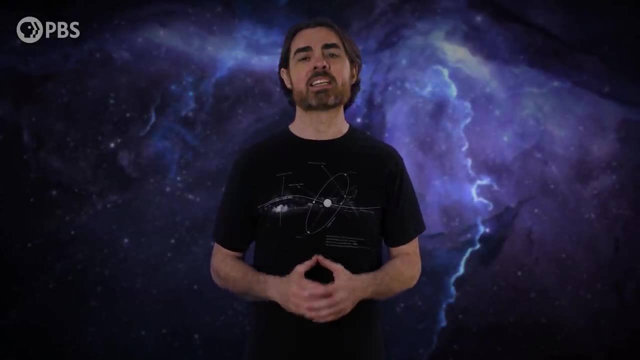 none of our intuitive explanations say that it should be deflected by gravity. So let's be smart and do what the smartest guy in the world did. Let's think about light in an entirely different way. Let's think about light in an entirely different way. 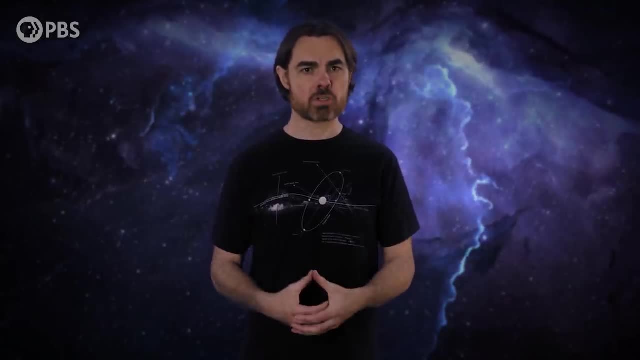 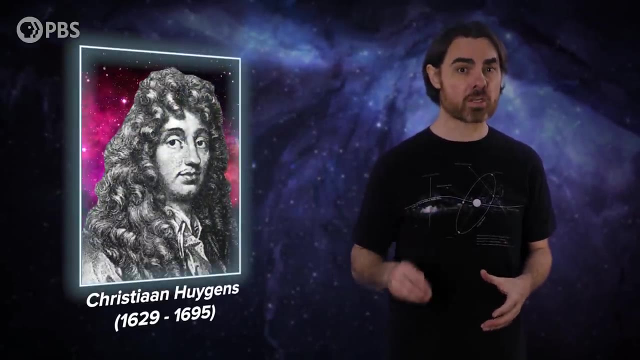 Let's think about light in an entirely different way. Energieogene was in the business of over turning the ideas of Newton, so it's not surprising that he turns to one of Newton's great rivals, the Dutch physicist Christiaan Huygens. 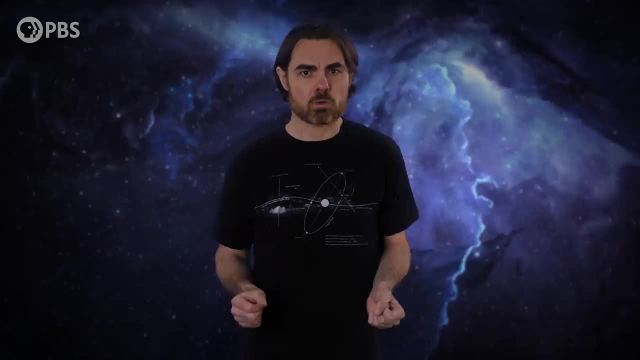 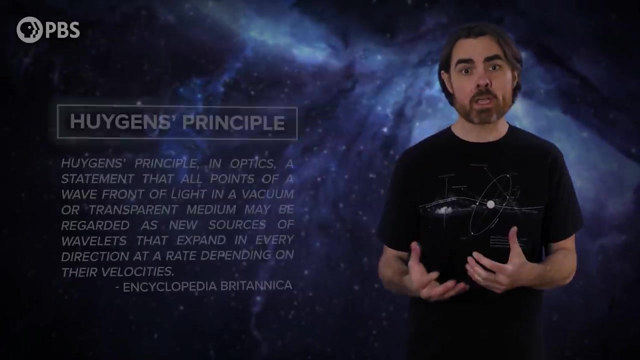 Disagreed with Newton on many things, including the idea that light is a particle. Huygens' wave theory of light advanced the field of optics enormously. A big part of that was his Huygens or Huygens- fractal principle. 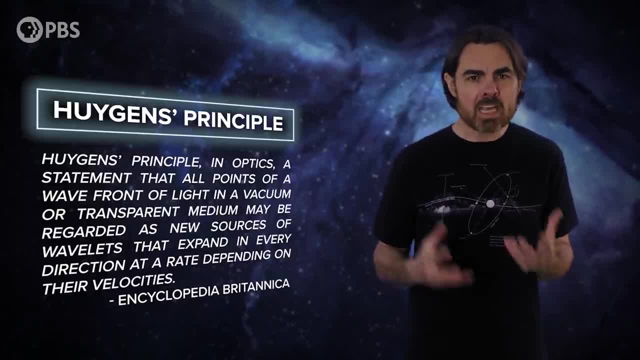 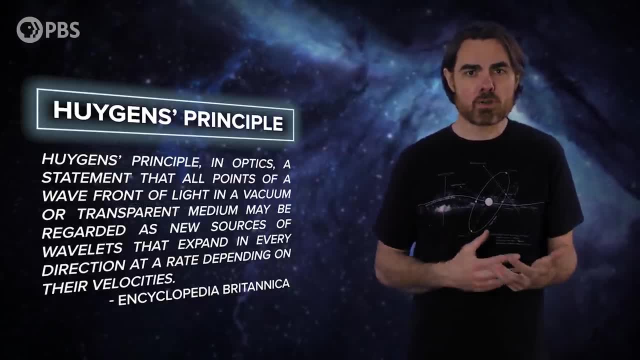 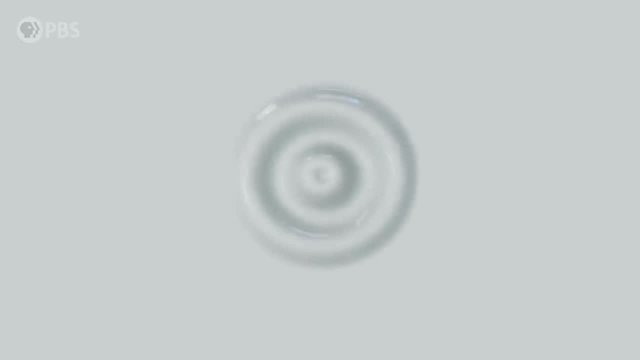 The idea is that any wave can be described as an infinite number of point-like oscillations, each of which produces new waves. The sum of all those waves perfectly describes the future evolution of the original wave. For example, imagine a single circular ripple on a pool of water. 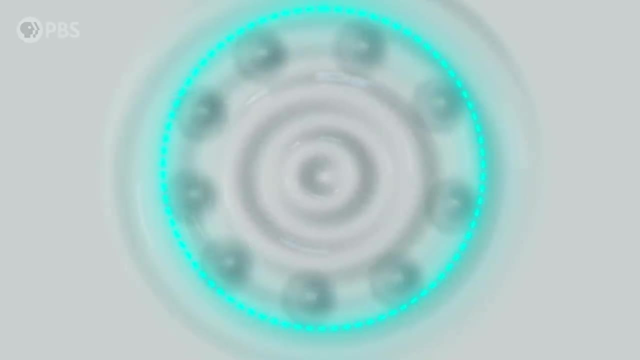 At any point in time. the expanding ripple can be thought of as an infinite number of sources of new circular ripples or wavelets. Those wavelets also expand outwards, but they cancel each other out everywhere except in the outward direction of the original ripple. 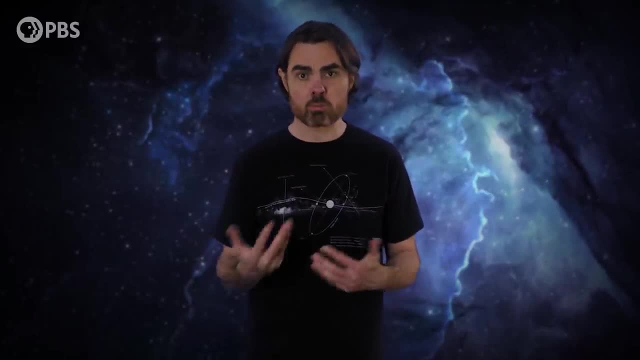 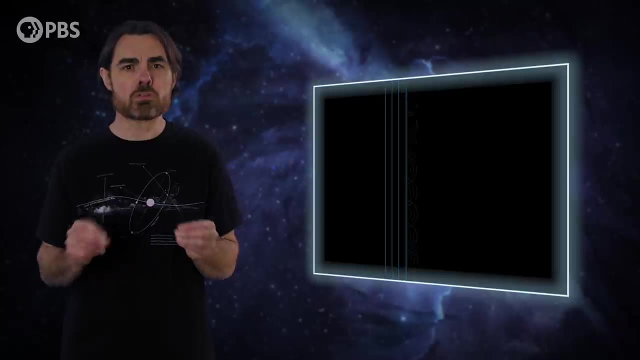 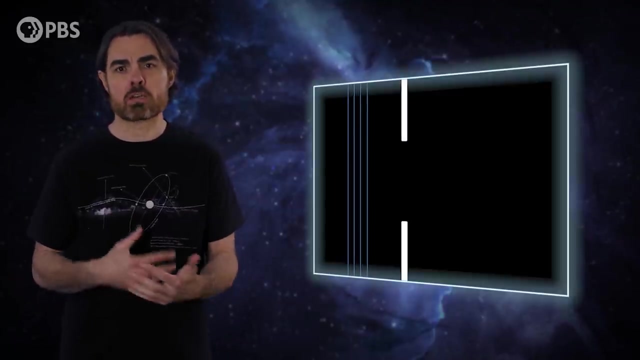 The result looks like the continuation of the original ripple. We can model light in the same way. A plane wave of light is just an infinite number of new sources of light that generate the next step in the plane wave. This explains why light can turn corners around opaque objects in the phenomenon of diffraction. 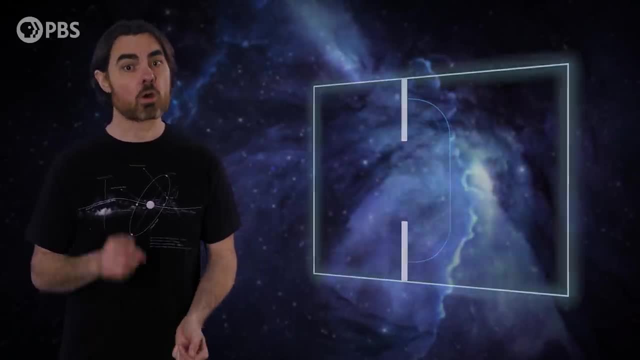 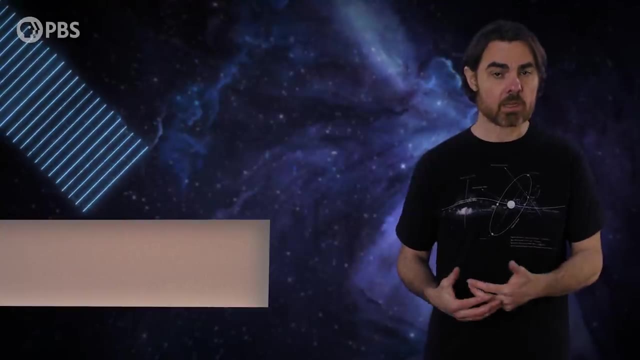 and why the path of light is bent when passing between substances. Refraction: Our plane wave reaches the boundary to a new medium. It's the same with the slower speed of light. If it arrives at some angle, then the next set of wavelets forming at the boundary will 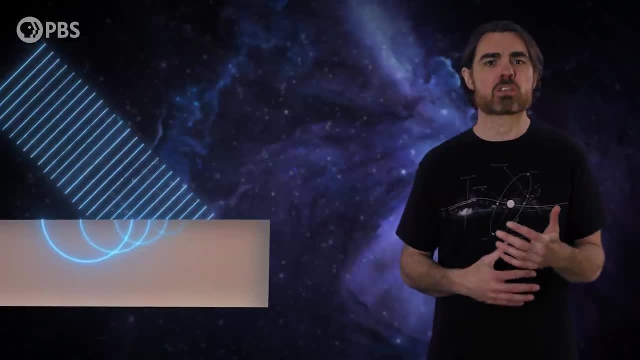 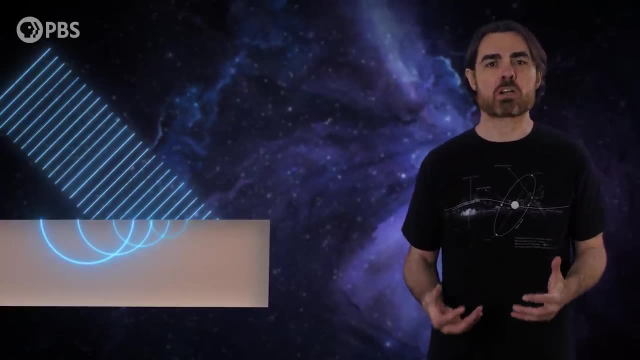 be more closely packed together. The fronts of those ripples don't travel as far in the time it takes to make a new wavelet. So now, if we connect the wavelets to reconstruct the overall wave front, we see that the path of light has bent. 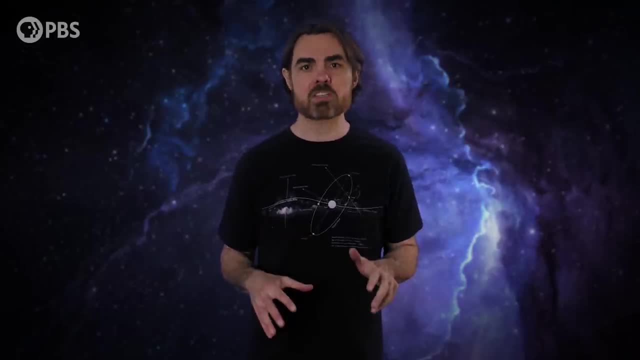 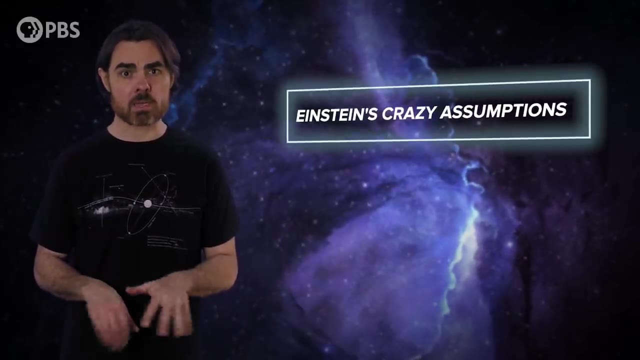 So that's refraction, But in a sense light gets refracted by gravitational fields, Or at least you can model it that way. You just need two completely crazy assumptions: First, that light acts like a very classical 17th century-style plane wave. so you can. 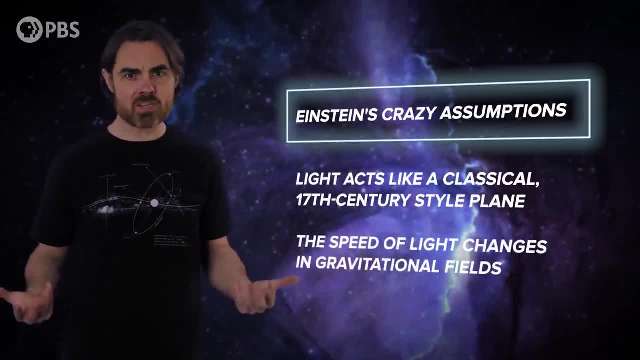 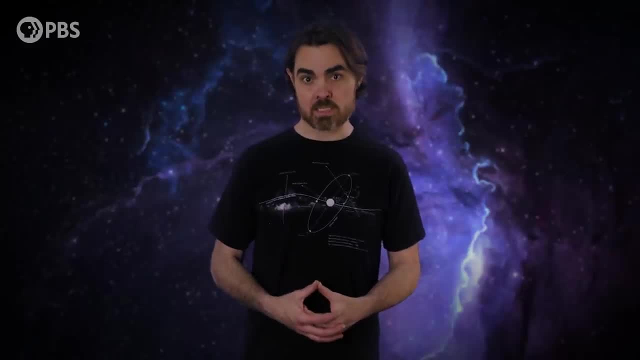 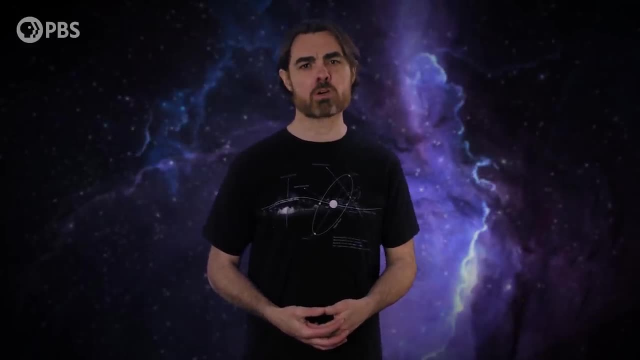 use Huygens' principle, And also that the speed of light changes in gravitational fields, which sounds counter to everything I've told you. But this is exactly what Einstein did. Let me explain why this isn't so crazy. after all, As you might expect from a theory called relativity, it's not just about relativity. It's also about the speed of light changing in gravitational fields, which sounds counter to everything I've told you. But this is exactly what Einstein did. Let me explain why this isn't so crazy, after all. First, that light acts like a very classical 17th century-style plane wave, which sounds counter to everything I've told you. 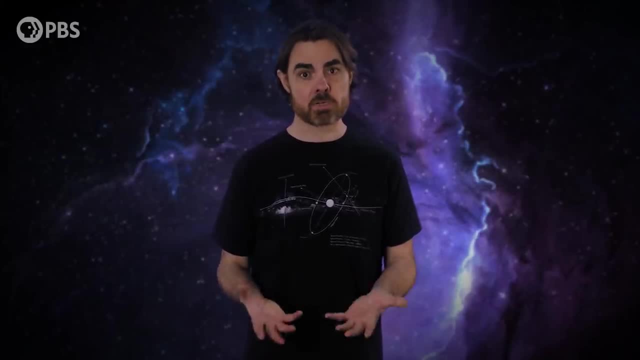 And also that the speed of light changing in gravitational fields, which sounds counter to everything I've told you, And also that the speed of light changing in gravitational fields, which sounds counter to everything I've told you. The only thing that's not relative is the speed of light. 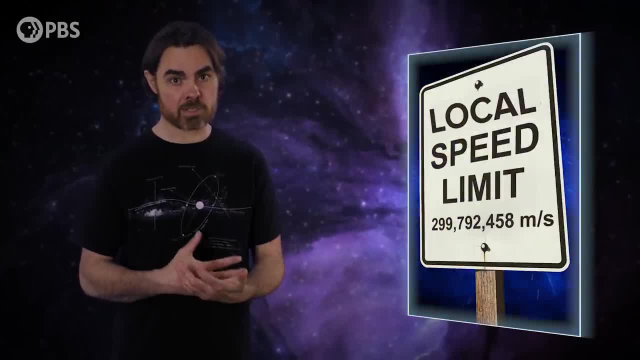 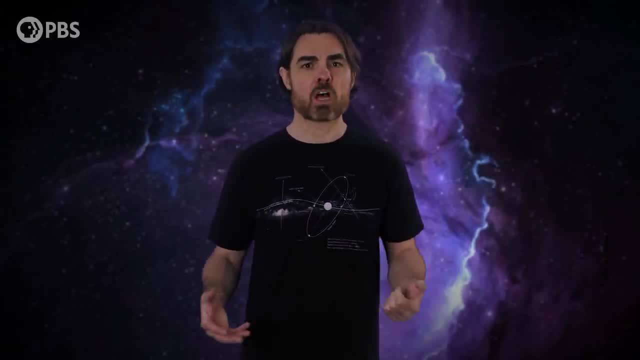 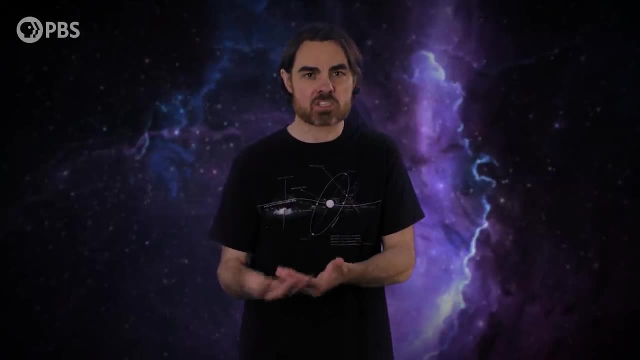 Everyone observes the same local speed of light in a vacuum. But notice that I said local speed of light. That means everyone measures the same speed of light passing through their own local patch of space. But viewed from a distance, the speed of light can at least appear to change. 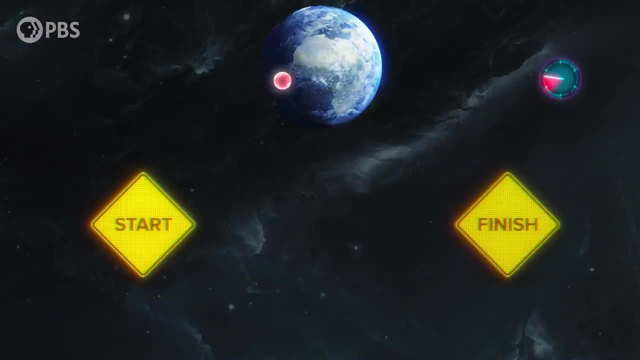 Ok, imagine you're looking at the Earth from a distance. A photon passes by and the amount of time it takes to reach it is only one in a thousand square meters. But if you look at the Earth from a distance, it's only the distance from the Earth. 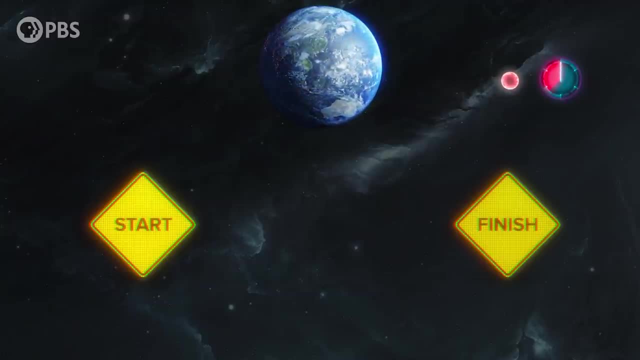 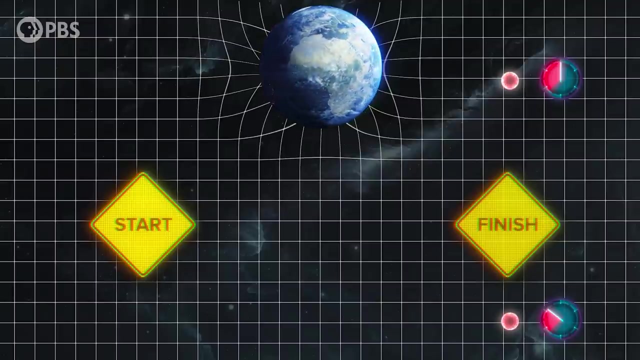 takes to cross that space is larger than if Earth wasn't there. That's because of two effects: Your clock is ticking faster than clocks in the Earth's gravitational field And space within the gravitational field is stretched. The photon has further to travel through a region of slowed time, and both of these effects conspire in the same direction: to slow the apparent speed of light. Of course, for someone actually inside the gravitational field, the photon is still traveling at the speed of light as it whizzes past them. And even if this change in velocity isn't real, it's enough to let us use Huygens'. 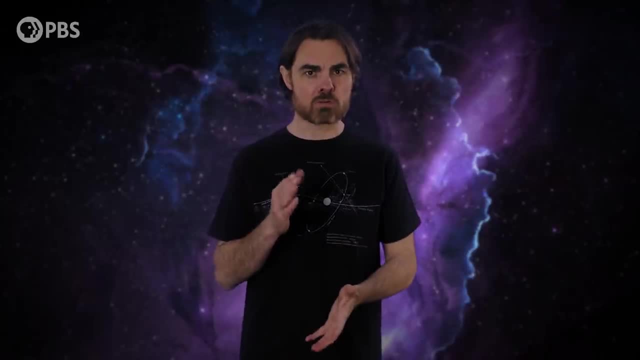 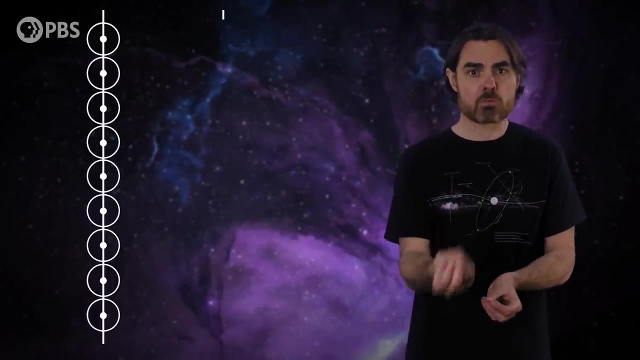 principle. At each location perpendicular to a gravitational field, the wavefront of light can be thought of as a vertical column of new wavelets. But for you, tracking this from a distance, the effect of speed of light decreases downwards because time slows and space stretches.